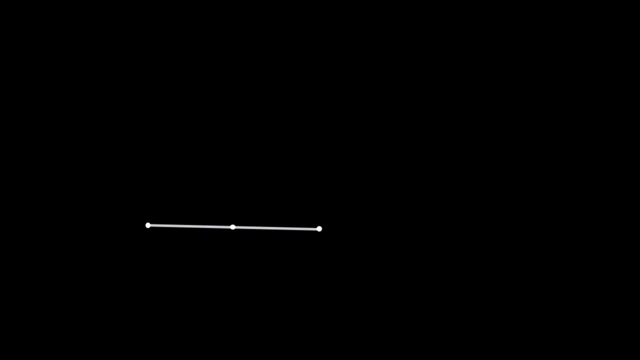 So we can get the midpoint of a segment. In Converse, If we know the midpoint of a segment, Can we get a parallel segment from a free point in the plane? Yes, We can prove it. Just form the diagram like this: 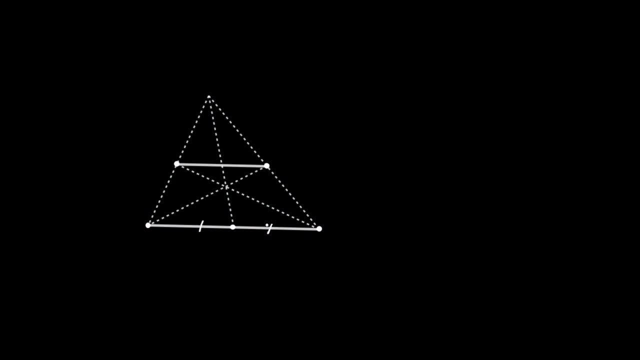 Because this two parts equal. Extend this segment, Make them equal. Now we get a parallelogram. We can prove two white segments are parallel. Now we get two conclusions in same plane. One is we can get midpoint. refer to a parallel segment. 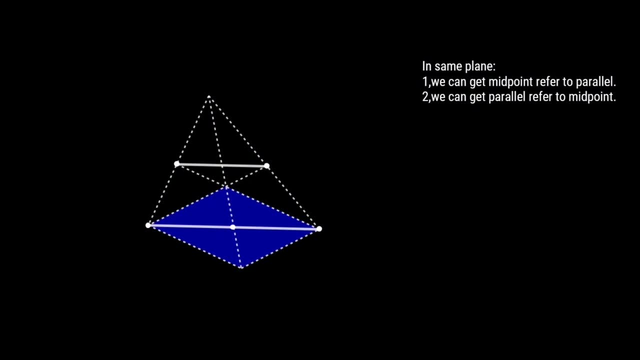 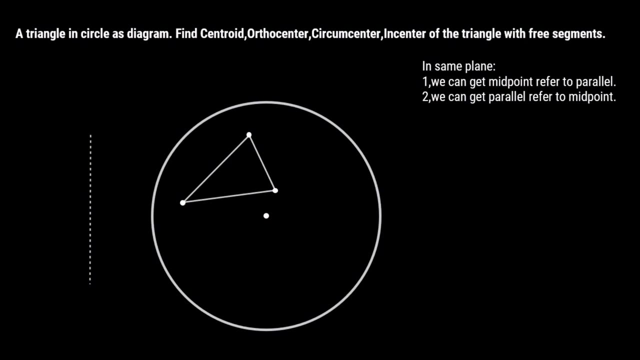 Other is we can get parallel segment. refer to midpoint. Let's recall to the problem: Connect center point of circle and a vertex of triangle, We get a diameter. We can get a parallel segment from this conclusion If we connect points of four points of parallel chords. 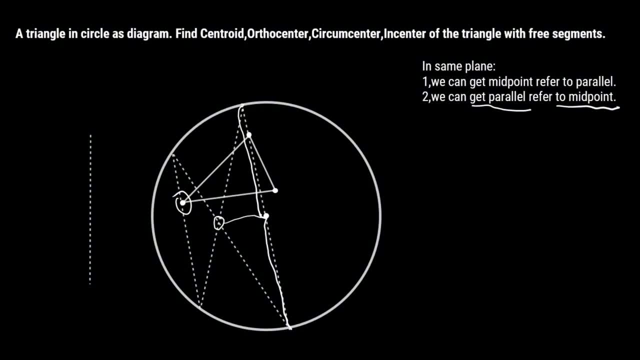 We get a crossed point, Connect to the center point. We can get another diameter which perpendicular to diameter each other, Because this two diameter divided and perpendicular each other. We can form a rectangle from this conclusion If we connect two points of parallel. 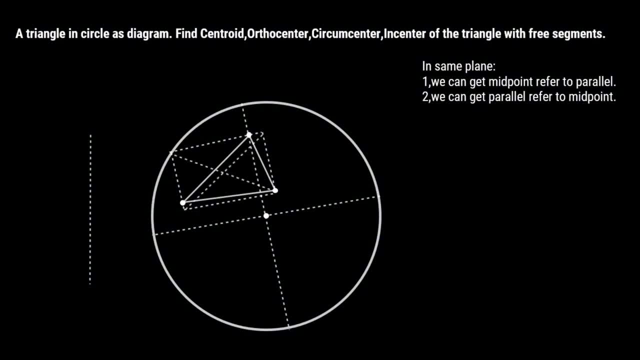 If we connect the diagonals of rectangle We can get the center point of rectangle, Make parallel segments through the center of rectangle, We can get two midpoint of the side in original triangle. In fact, We get another important conclusion, That is: 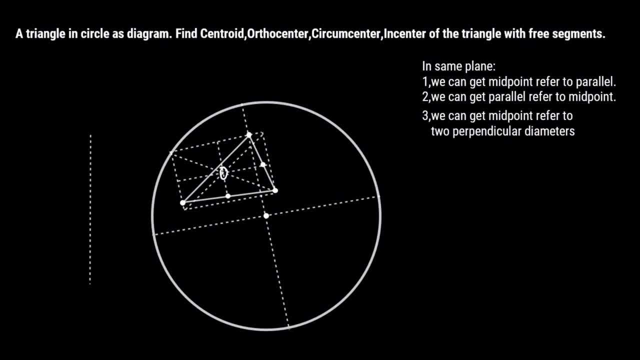 In the plane We can get midpoint refer to two perpendicular diameters in circle. So we can get midpoint of segment directly in this diagram. Now we can get the centroid of triangle. The centroid of a triangle is the intersection of the three medians. 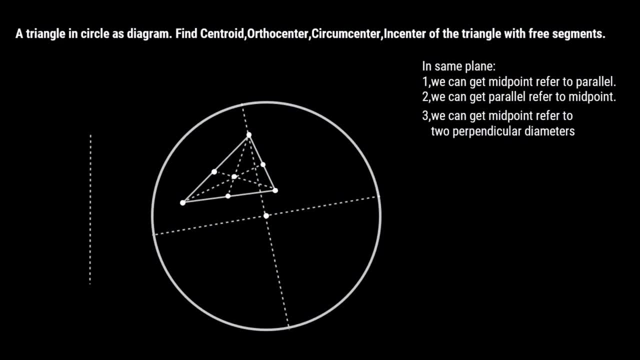 This is the centroid of triangle. This is the centroid of triangle. This is the centroid of triangle. Then let's go ahead and find the orthocenter of the triangle. The orthocenter of a triangle is the point of intersection of its altitudes. 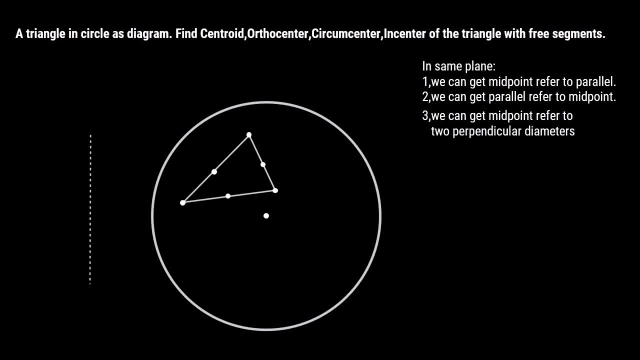 How to get the altitudes in this diagram. Let's extend one side of triangle and intersect to the circle, Because diameter intent to a right angle, So we can find a right angle. We can find midpoint from this conclusion And make a parallel segment through this segment. 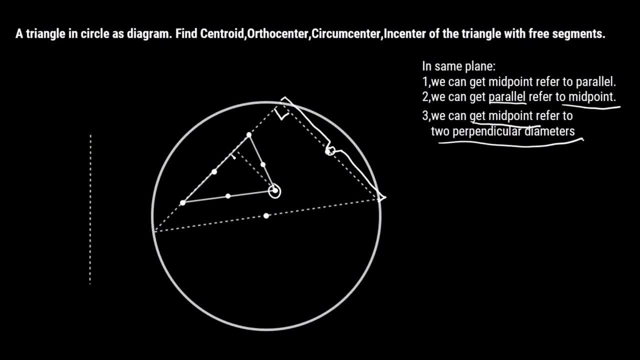 So we get the first altitudes in the triangle. We can repeat the steps and get the second altitude. Now we get the orthocenter of the triangle. Then let's find the circumcenter. The circumcenter of a triangle is the perpendicular bisectors of the sides intersected. 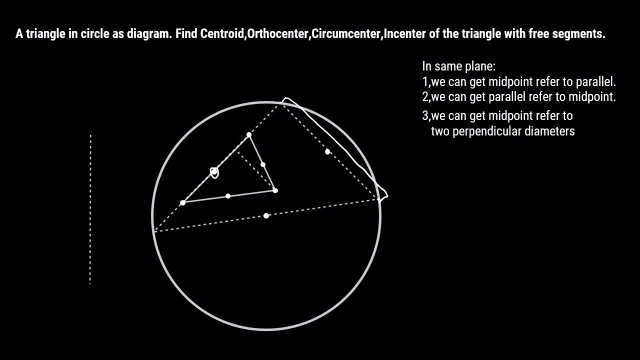 We just need to make a parallel segment through this midpoint to the leg of right triangle And repeat to the steps We can get the circumcenter of triangle. The last one is inckenter of triangle, And center is the point which the bisectors of the interior angles intersect.